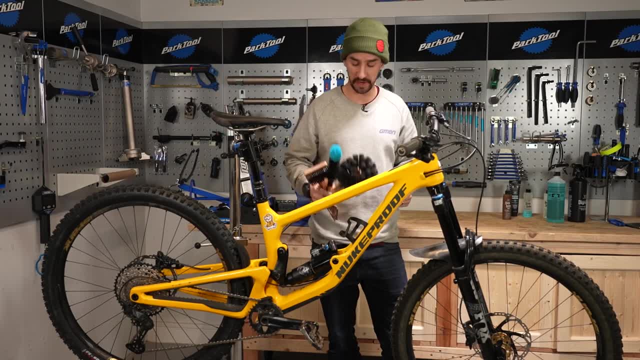 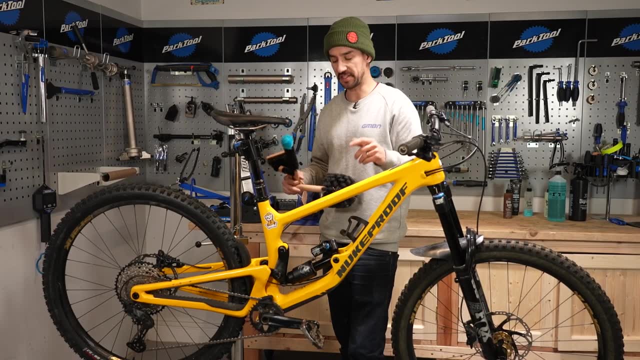 A nice selection of brushes are really going to help you get into your bike and clean it out. Also, it sort of helps you especially getting if you've got a full-spension bike. getting into the linkage with a brush is going to save you firing too much water down into there. 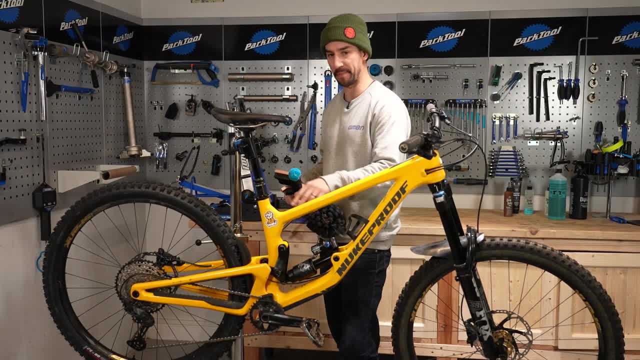 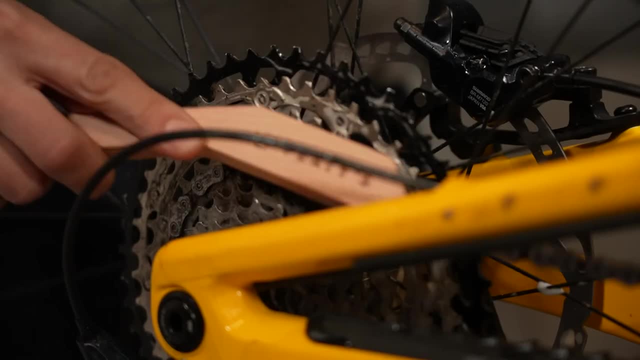 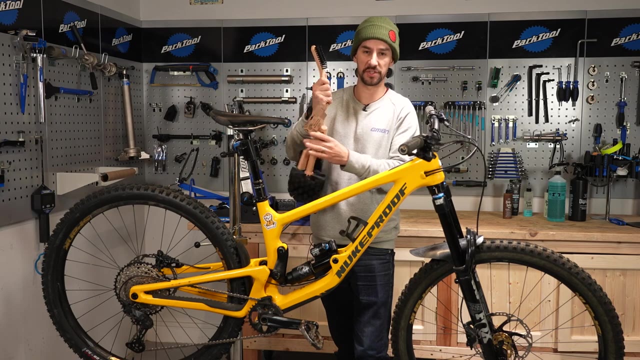 Also, I'll keep a separate brush just for the drivetrain, because that's going to get oily. I don't want to use that anywhere near my disc, so I'll use that around non-oily places and save one for just that mucky application. 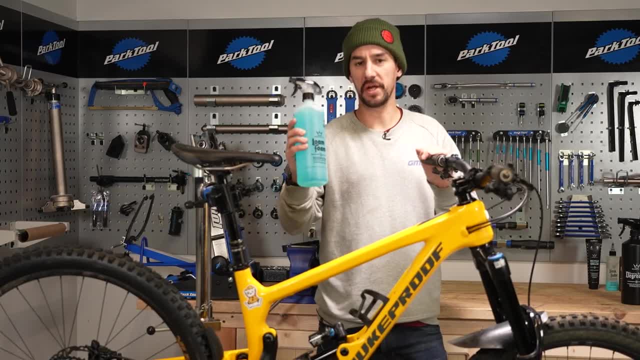 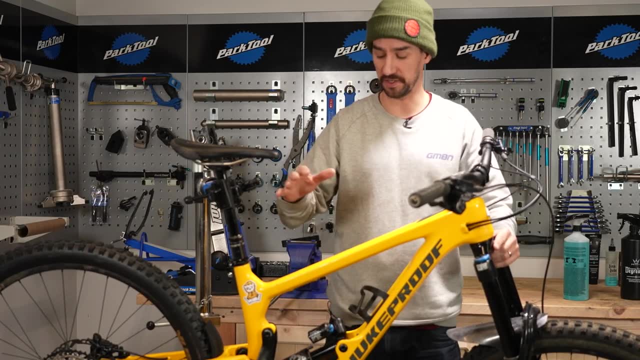 where you don't want to get it on any other part of your bike. Washing your bike after muddy rides and also making sure that you're putting it away dry is going to extend the life of your bike by such a big margin If you're just riding it, keeping it dirty. 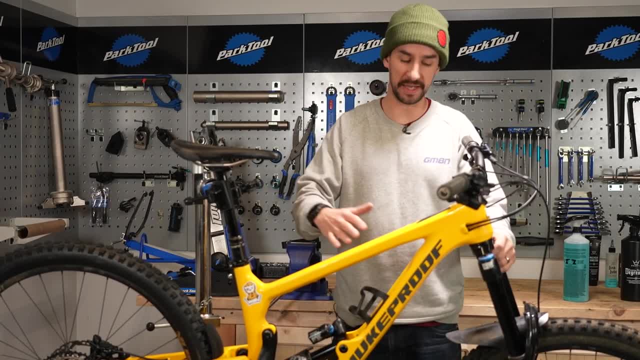 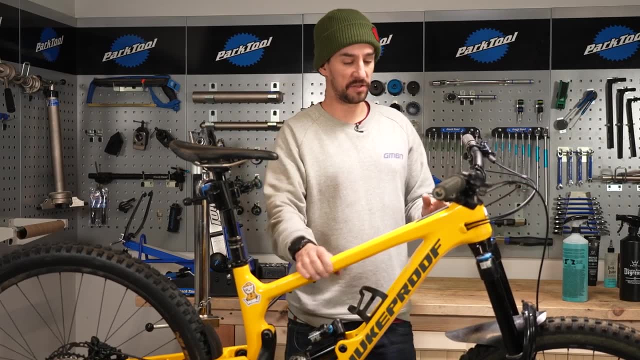 and then riding it again. things will wear out, So I'll always make sure as well. once I've washed it, I've got a big old towel that I'll use to dry everything off, and then I'll sort of get into what needs doing next. 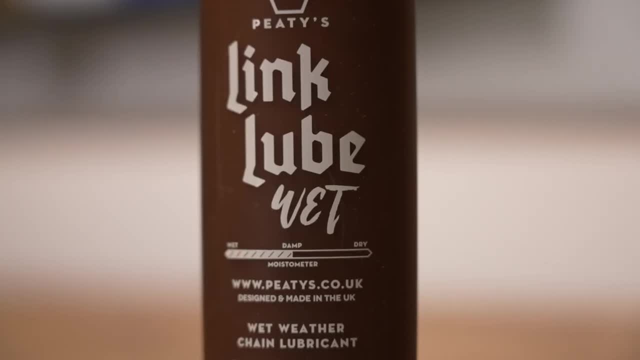 So often in winter, if you're using the proper lube- so wet lube- it's got special ingredients in there so it'll stick to your chain. So if you're riding through puddles it doesn't get washed off. 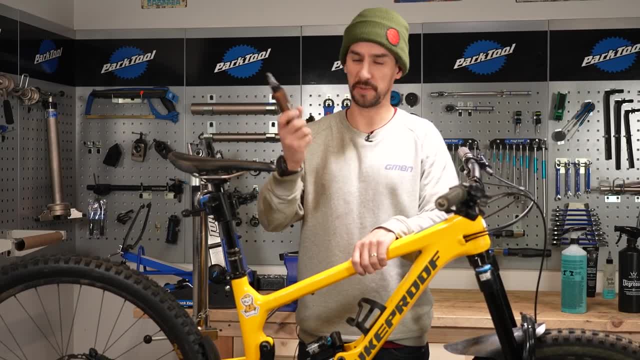 Like a dry lube will. in summertime great for that, but in winter, especially in the UK, if you're riding somewhere really wet, then get some of that stuff on. But the problem with that is it is thicker and it'll stick to your chain. 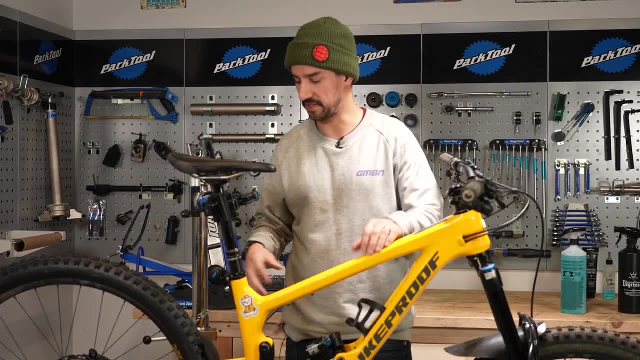 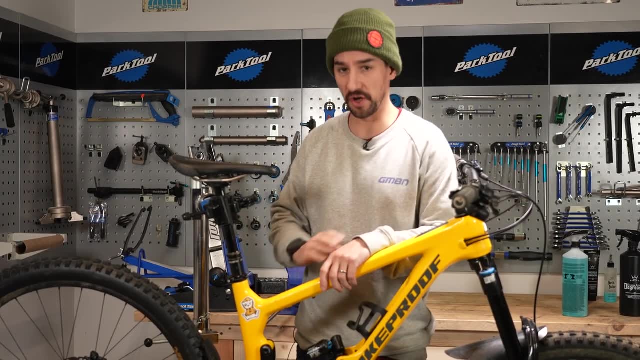 and then if you don't clean your bike, it basically turns into grinding paste. You'll see if your chain gets really black. All that mud and grit and sand- whatever that's sticking to your chain- is then grinding into everything. So your cassette and your chain ring. 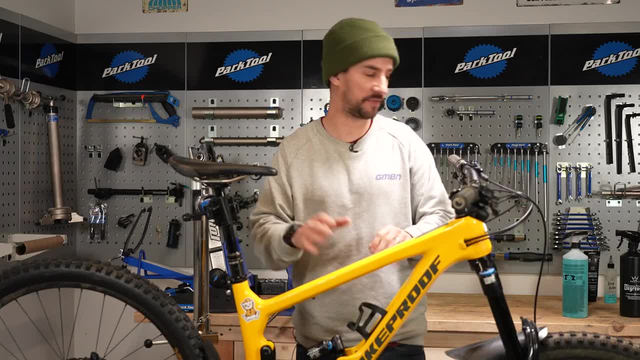 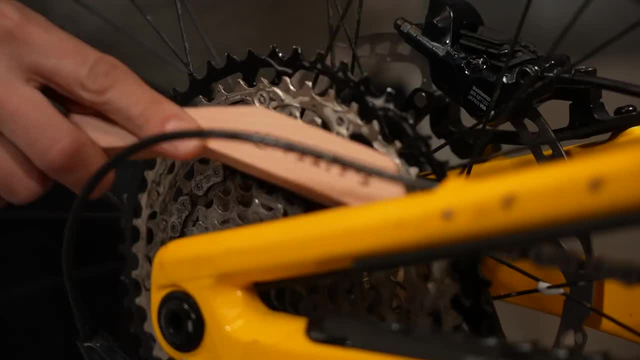 and it's wearing them away and that will wear your stuff out so much faster. So that's when it's time in winter to get the degreaser out as well. So this is specially formulated to spray onto drivetrains. 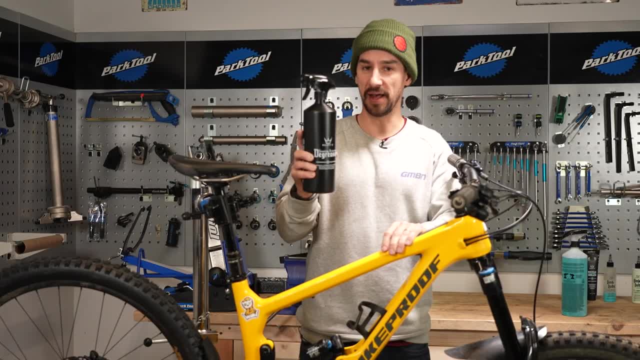 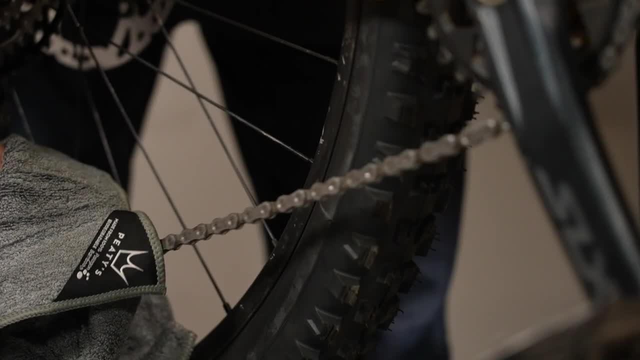 It's not going to start ruining any other parts of your bike. It will get in there. it will get your old lube off, make it nice and clean, and that's when, again, I'll dry that chain out. make sure the whole bike's dry. 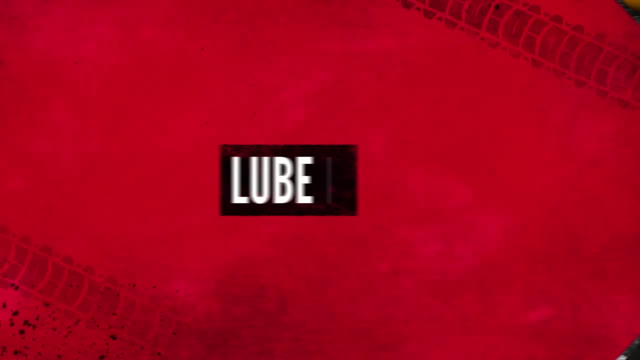 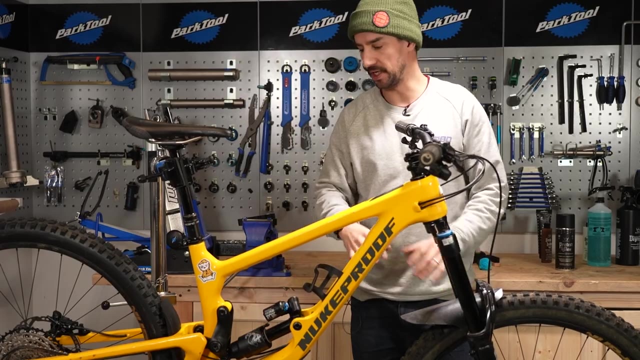 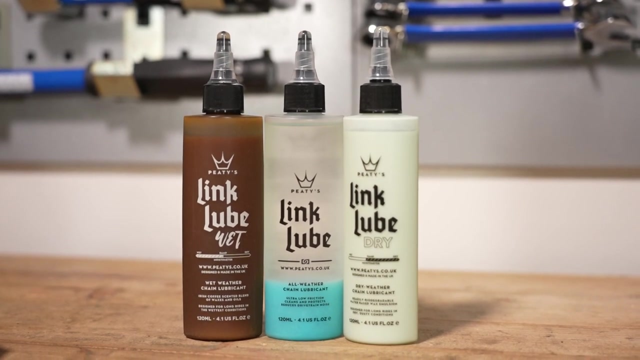 and then I can start re-lubing it ready for the next ride. So once the bike is clean, it's time to lube it up, Like I said, picking the right chain lube for the choice of conditions. You've got dry, wet or even all-weather chain lubricant. 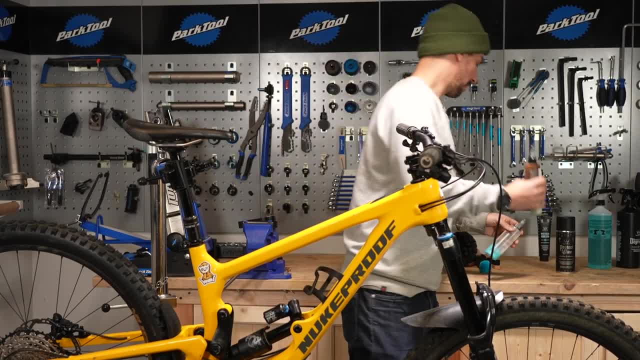 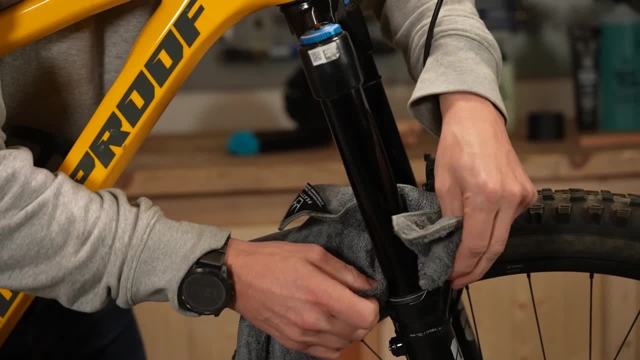 so that does a bit of everything. so that's quite an interesting one. Also, making sure that your shock and fork are nice and clean Round the seals. I'll double-check those. I'll normally get rag and run it round here as well. 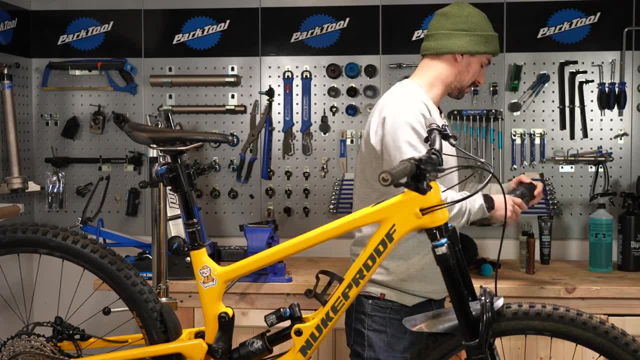 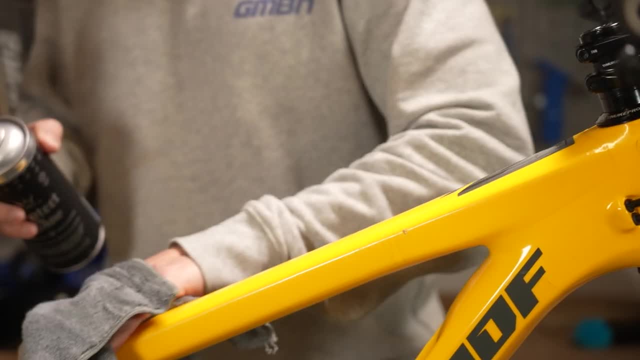 to make sure they are super clean And then get some silicone spray. So this is stuff that I'll actually spray onto a rag and then go over the bike with a rag, Rather than spraying this too much on the bike if you get this on your disc brakes. 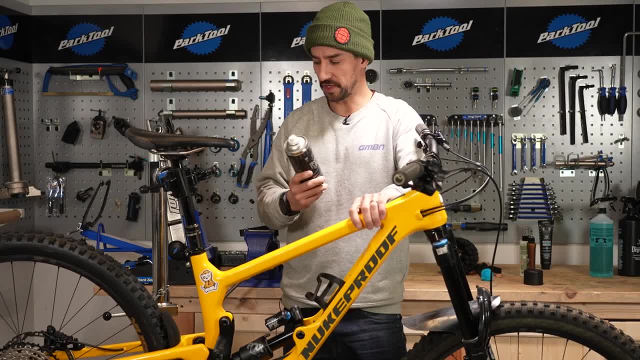 it just ruins them. it'll stop them from working completely. Sometimes you can burn it off. I've done that quite a few times. If you get a blowtorch, it's not great, or if you've got a brake, it's not great. 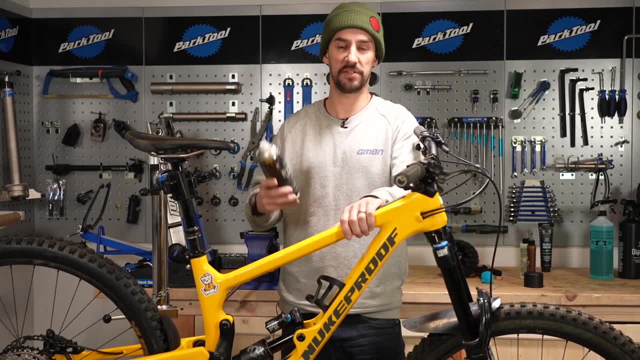 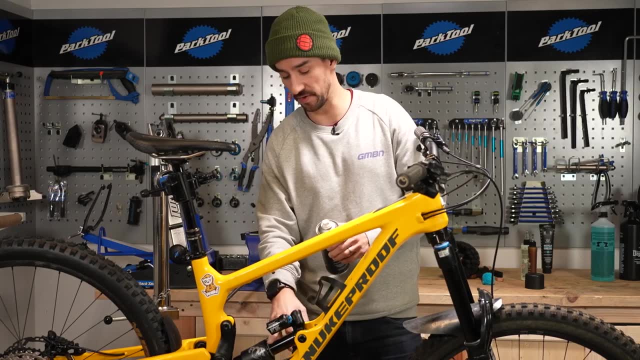 But you probably need some disc brake cleaner as well. But it's obviously better just to not get it on there in the first place. So we'll get this on the frame makes the bike super nice and shiny, but also make sure I'm getting this on the shock. 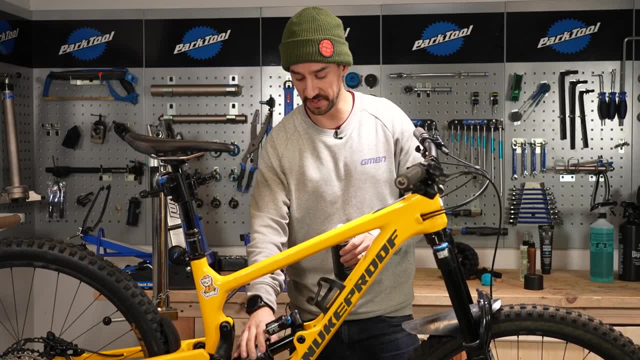 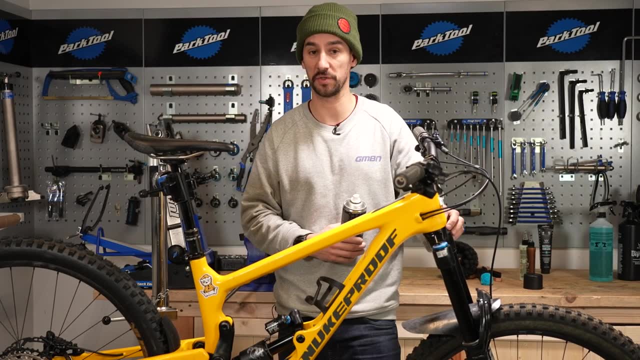 and the fork. It's going to help them keep nice and smooth, Same as the chain. If they're dirty, you're just pushing dirt and grit up and down there and they're expensive. You need to start replacing stanchions on your suspension. 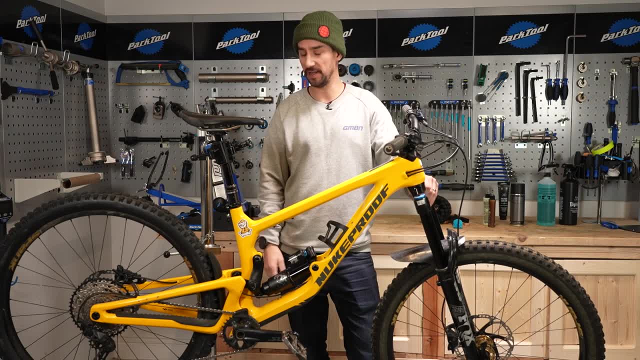 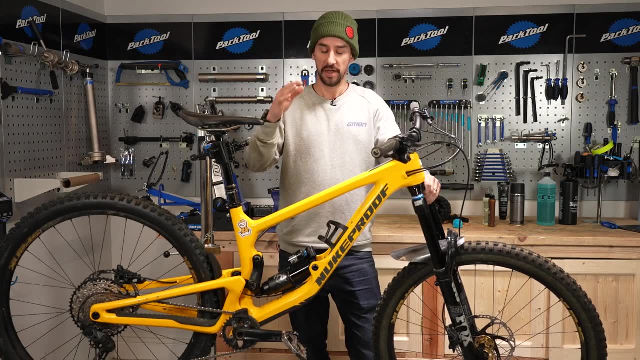 Where you keep your bike is also probably going to determine its life longevity a bit as well. So if you're lucky enough, like me, to have an indoor garage that's actually heated, it's great. Obviously, I'll make sure my bike is dry. 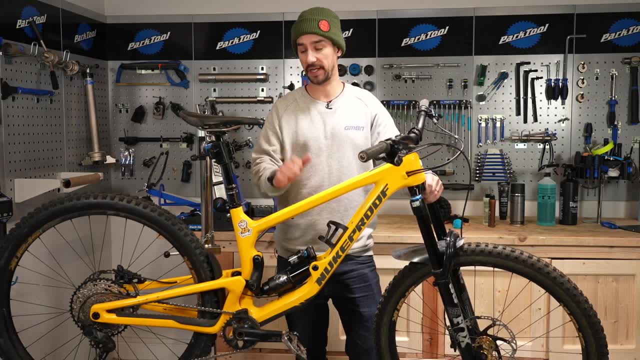 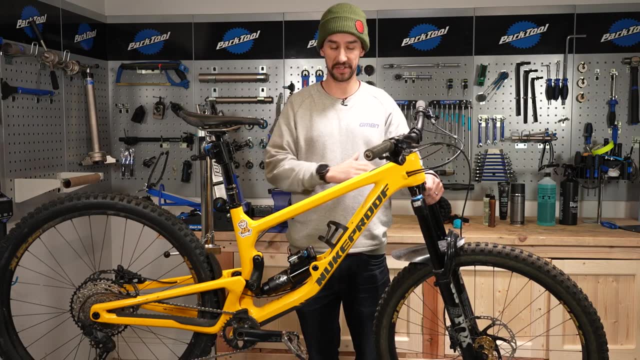 because if you're putting a wet bike into somewhere that's heated, it's going to get rusty really quick, But if you're keeping it outside in the shed it's not ideal. I have had this before. I've got an outside garage. 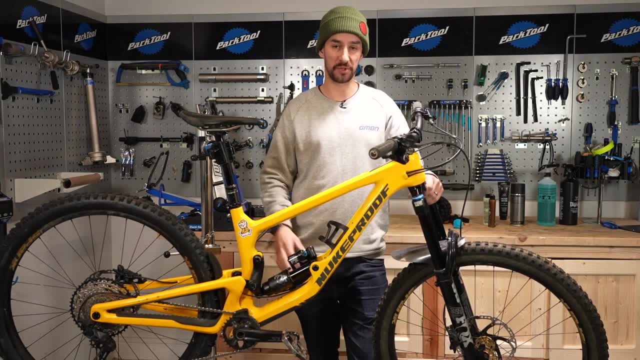 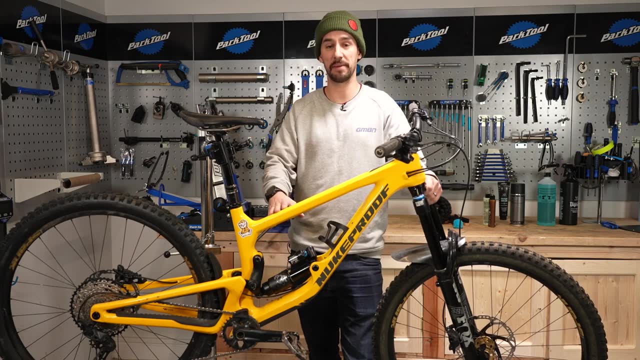 and bikes have got a bit damp and it will start rusting up your chain in there. So hopefully you can keep your bike nice and dry and warm. If not, maybe we're thinking about covering it up so it doesn't get damp. 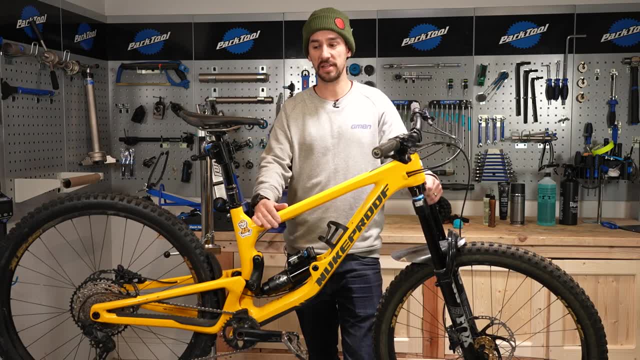 inside a garage. I guess this is something that you can't really alter. Either you've got a nice garage or you haven't, But definitely if you can keep it nice and dry and warm, your bike is going to last that little bit longer. 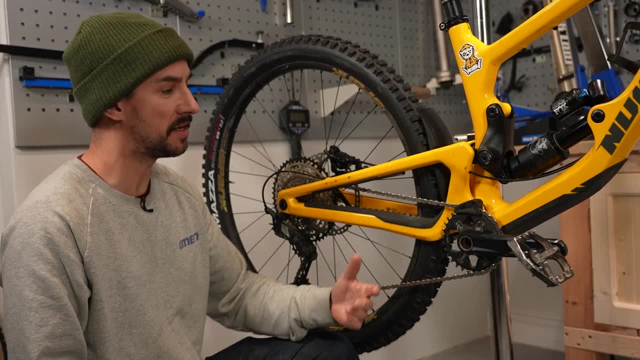 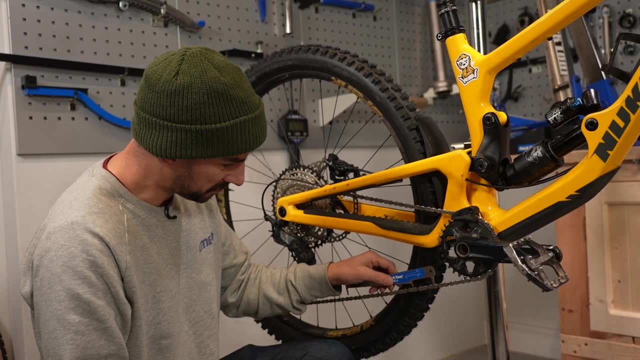 So you've got chain and cassette doing a lot of the dirty work on your bike. Obviously, keeping it clean and lubing is great, but it's also worth checking it as well. I hate replacing drivetrains. It's like one of those things. it's expensive. 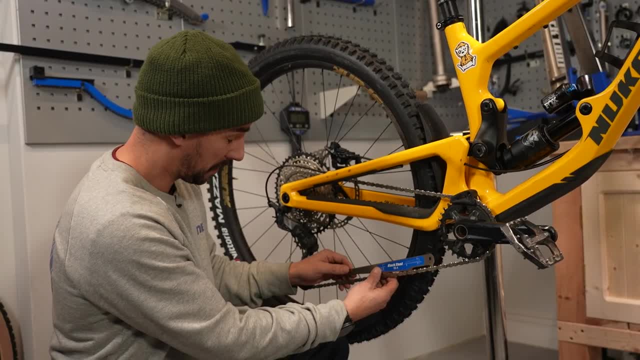 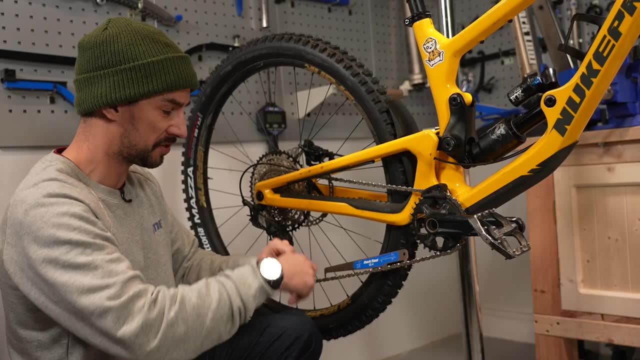 and your bike doesn't feel any different for doing it, But hopefully it'll shift a little bit for anything. But what we can do is get a chain checker like this, So this will check how much your chain has stretched. So when they get worn out, they get super floppy. 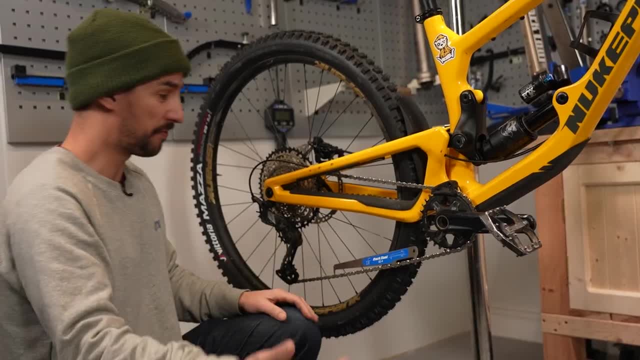 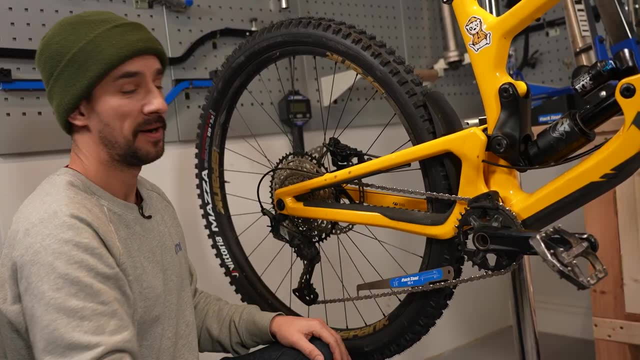 but they'll also stretch and get longer, And if they get too far, obviously it'll start slipping, and that's the time when you have to replace it all. So you'll need a chain and cassette, and possibly even a chain ring as well. 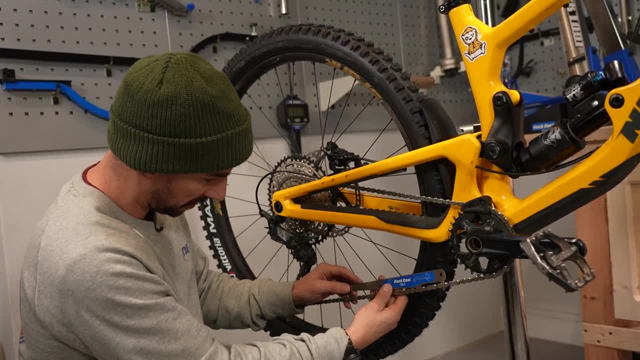 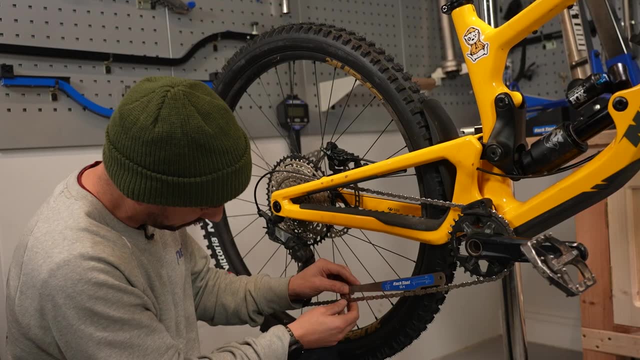 And that's when it gets expensive. So if you keep an eye on how much your chain is wearing when it's checked, it goes up to 0.5, and then, if it gets worse, this goes in further and goes up to 0.75. 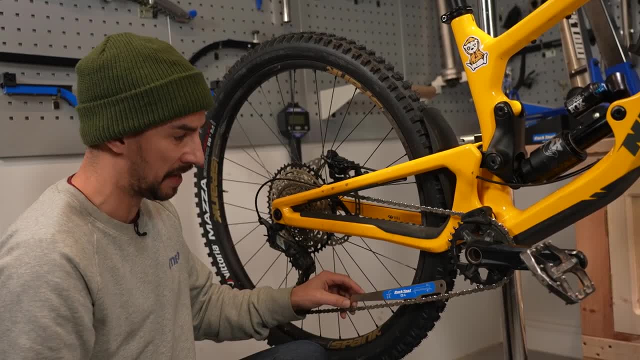 But if you replace your chain at around the 0.5 mark, then a new chain will go on to the old cassette and it'll work If it gets too worn up to the 0.75, if you put a new chain on. 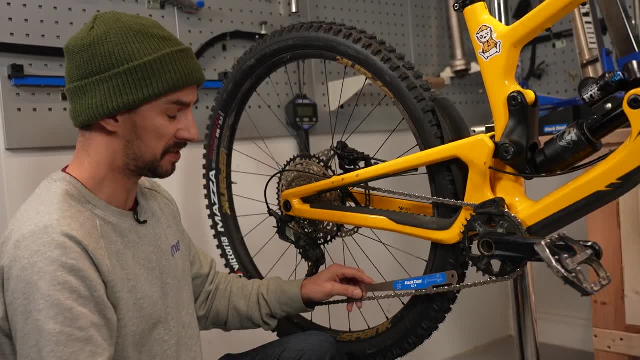 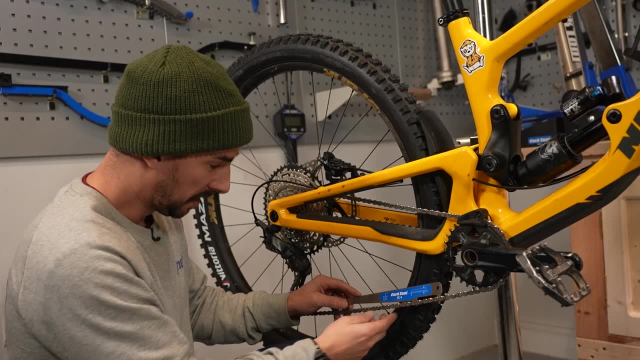 it'll just slip on the old cassette anyway, so you have to then go down a more expensive route. So if you're replacing chains more regularly, then you won't have to replace a lot. So you'll probably get two or three chains per cassette. 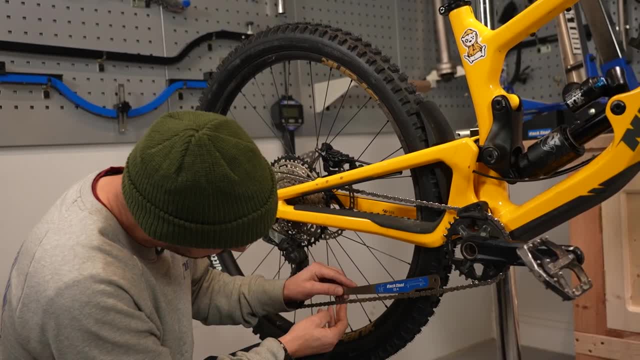 So just keep an eye on this. At the moment, I'm not even up to 0.5 yet. so this chain- I'm not even up to 0.5 yet, Although it looks a bit dirty. I need to clean it a bit. 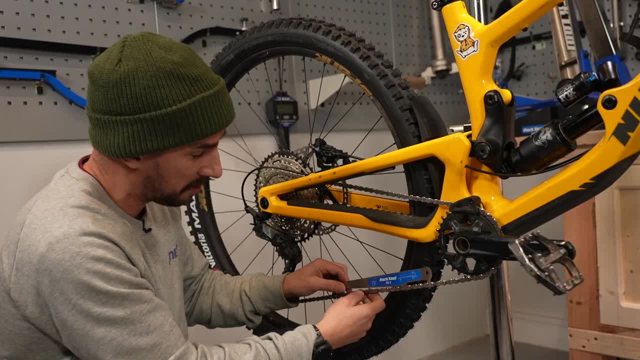 it's actually not worn at all yet, so I've got a decent amount of life left in this. Hopefully it'll last me all the rest of winter, because that's what I'll also do- is try and get it through the worst of winter. 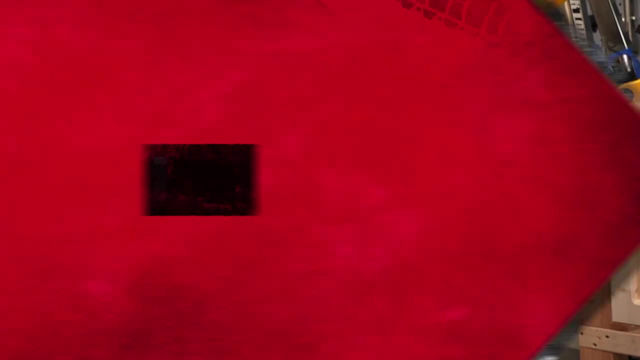 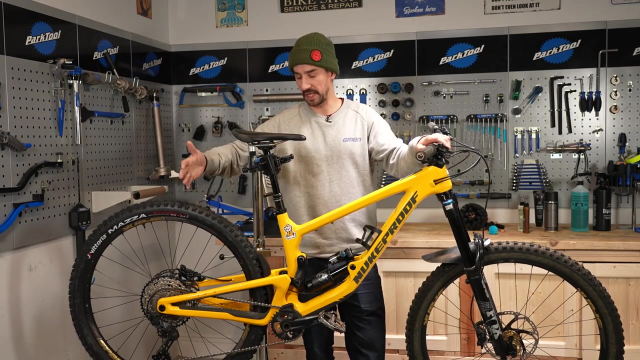 and then in summertime, don't feel so bad about sticking a new drivetrain on. Tyres are expensive, so I always think about trying to get the most out of them. I'll use a rear one, particularly until it's dying to death. 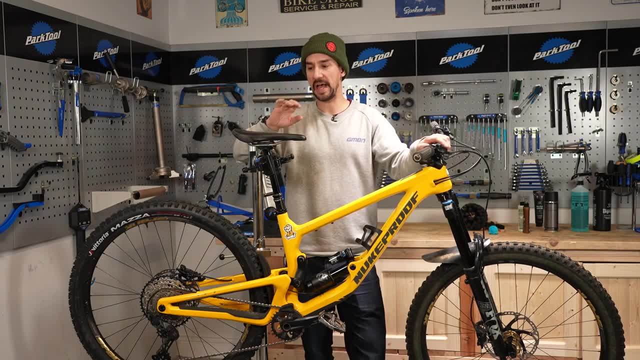 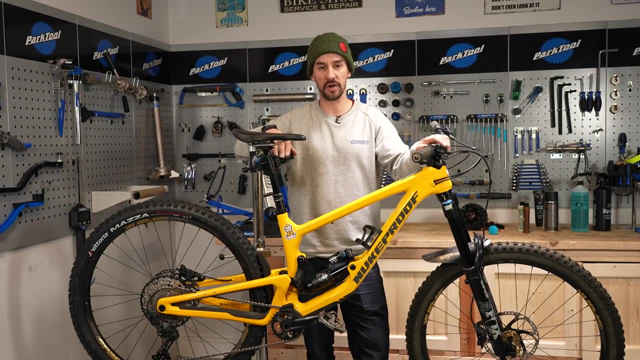 and the knobs are just going to be completely worn down. But also I'll err on the side of having a slightly too tougher, heavier tyre, Just because if it's too light, you're going to start ripping it if you're riding gnarly terrain. 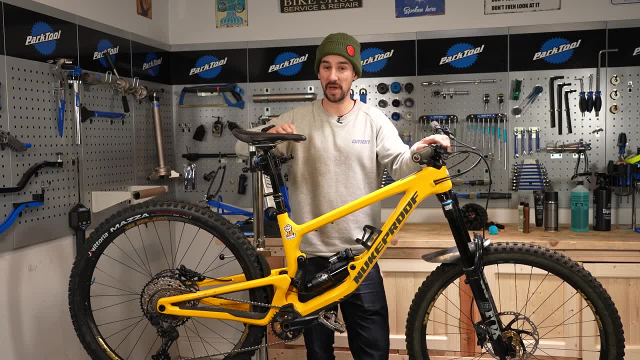 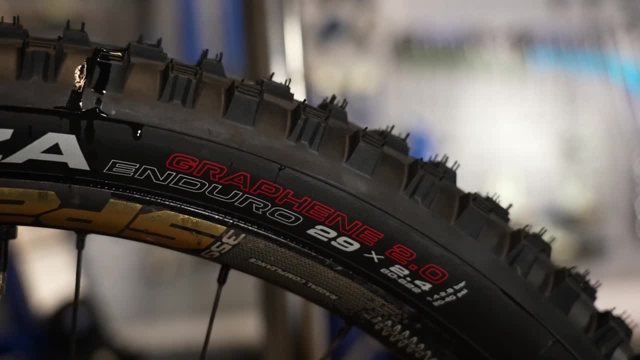 and then, yes, you can repair them to a certain degree, but it'll also wear out quicker as well. So on my Nukeproof Giga I've actually got a Vittoria Mazda Enduro build, so that's their toughest build on the rear. 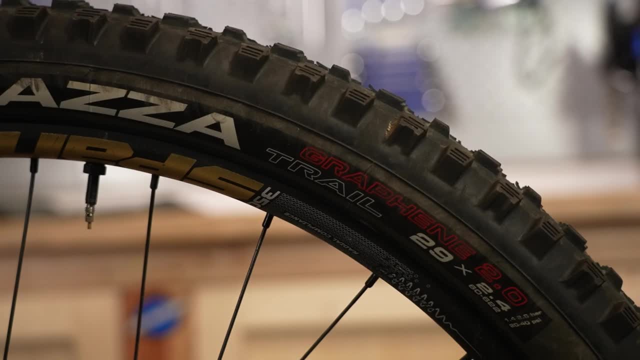 And then I've got a Trail up front: save a bit of weight and the front tyre doesn't take that much hammer. But on the rear, if I had a Trail tyre, I'd end up pushing it pretty hard, possibly rip it. 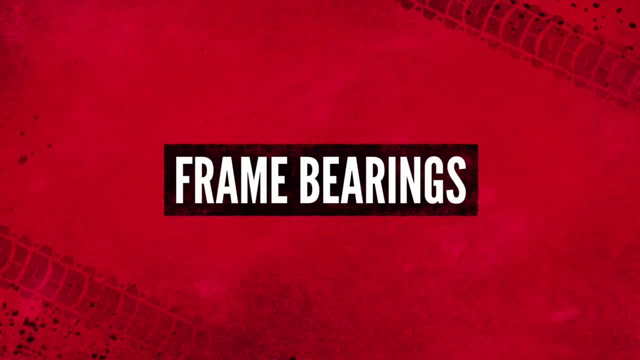 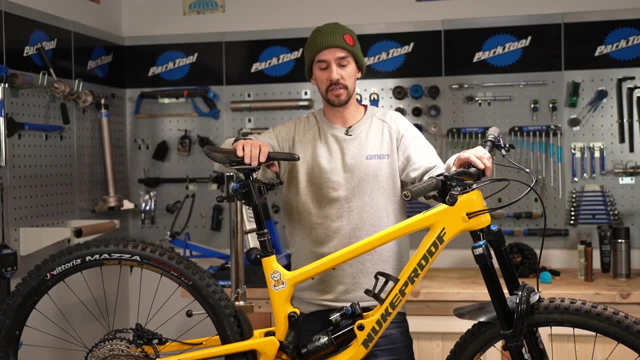 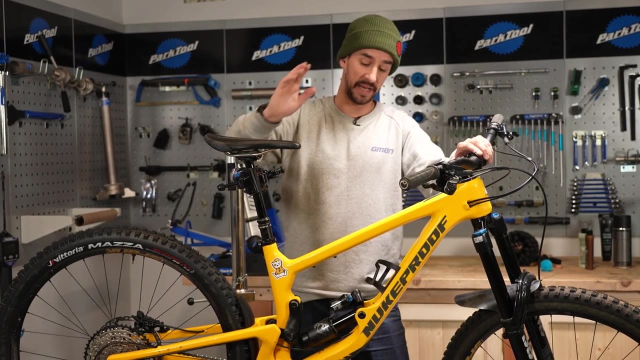 so I'd rather get my money's worth out of a slightly heavier tyre. Servicing your bike is obviously going to help it last longer, so make sure you've got a reasonably basic tool kit, and then you're going to need some lubricants. 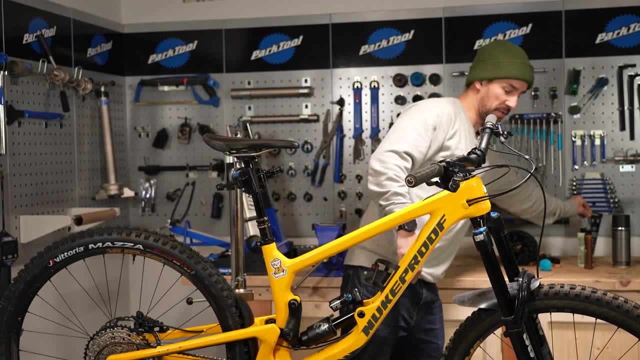 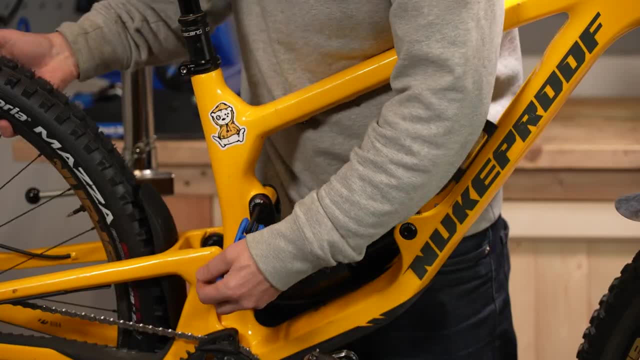 and greases and things like that, because I'm going to start digging into the moving parts of my bike. So on a full-spension bike, definitely during winter, I will take the pivots off. Have a look, You might feel that they're actually really smooth. 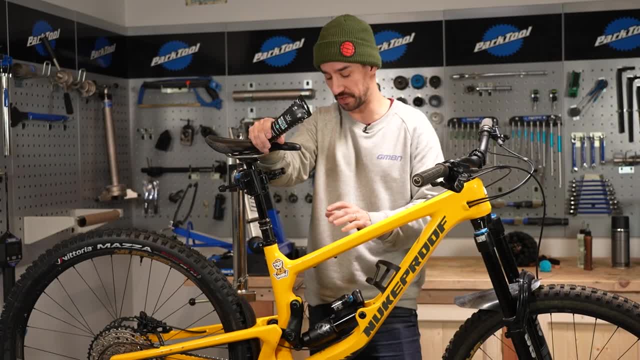 and they're dry in there because you've got really good seals now or you've been super careful not washing it. You might find that you can start taking them apart, cleaning them out and re-greasing them to help them last a bit longer. 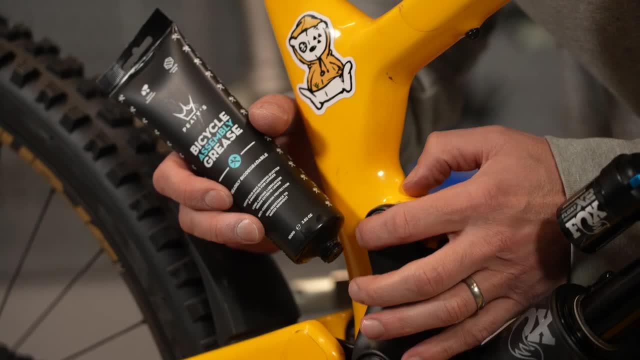 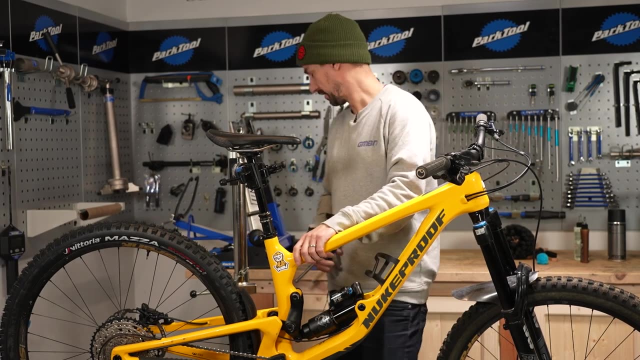 Even getting a bit of grease around the seals is going to stop water getting in there as well. So any sort of enthusiastic mechanic can do this. You don't need to be super into this and know exactly what you're doing. There's not much that can go really wrong with a bike. What I would say is just trying to keep up with the bike, so you don't need to be super into this and know exactly what you're doing. There's not much that can go really wrong with the bike. What I would say is just trying to keep up with the bike. 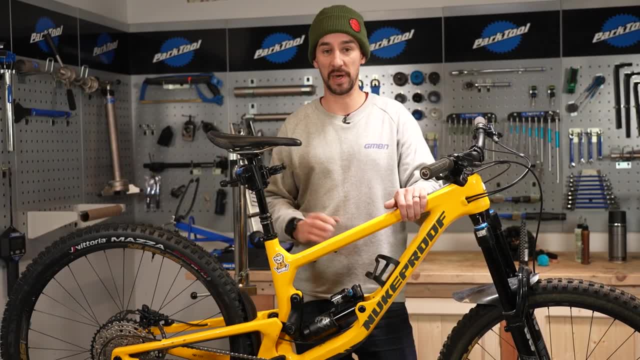 so you don't need to be super into this and know exactly what you're doing. What I would say is just trying to keep on top of that. Like I say, inspecting it fairly regularly is a way to know if it needs doing or not in the first place. 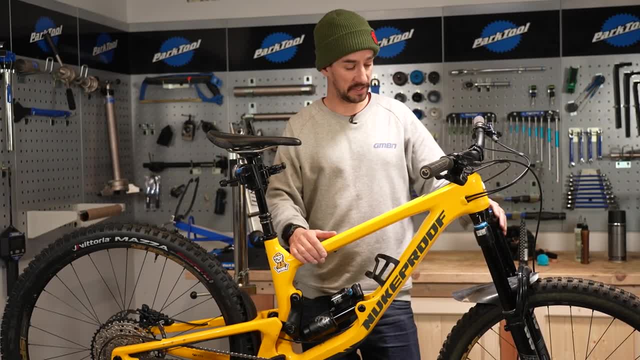 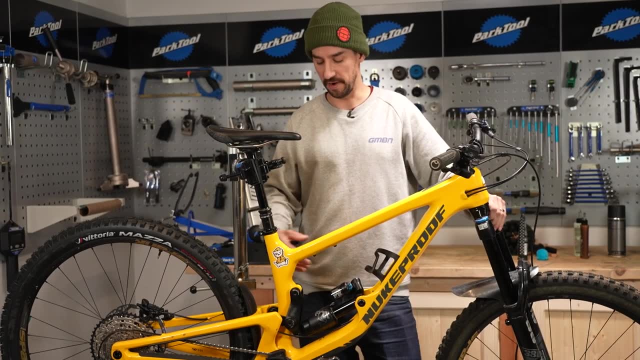 And then things that I don't do I will send off are a suspension if I feel like I need servicing. Also, there will be service intervals in these things. that is kind of worth looking into, Whereas, you know, pivots bearings. 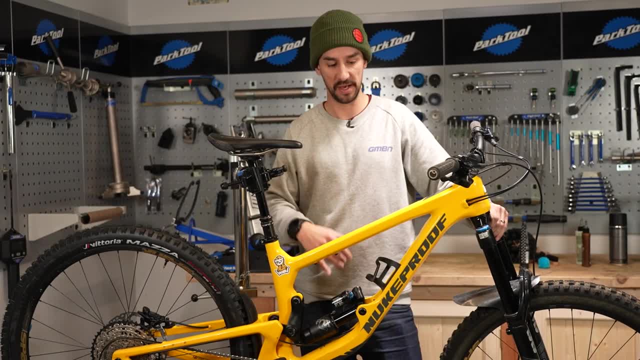 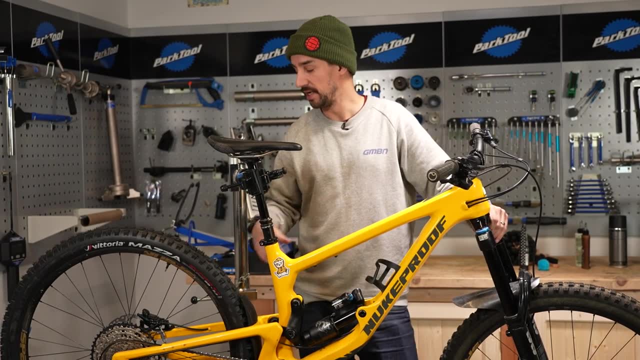 it's more about keeping an eye on yourself. These will have a number of hours, and then it's worth thinking about sending them off, getting serviced The rest of it. keep on top of yourself. Check out all your bearings, like your headset, your pivots. 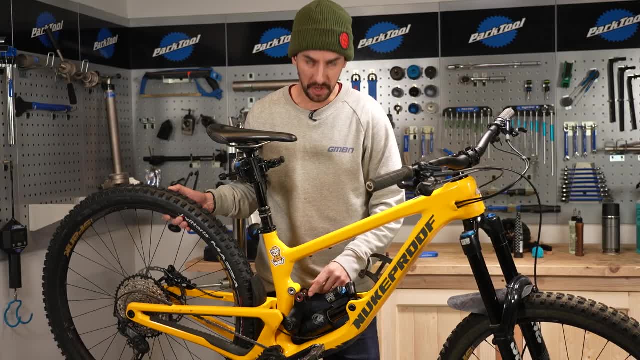 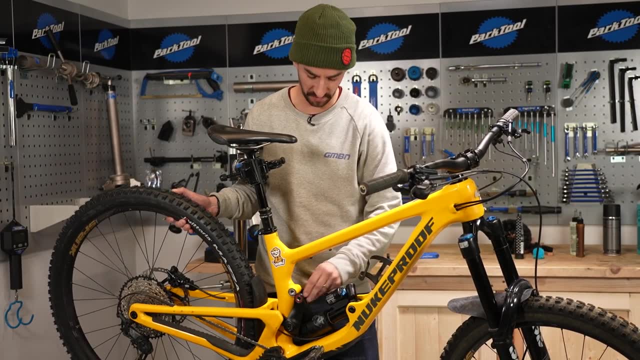 your wheel bearings- even your pedals, are pretty easy to service yourself. In my experience on sort of modern bikes, these frame bearings should last you a year, so a summer and then a hard winter's ride in UK conditions. These ones still feel nice and smooth actually. 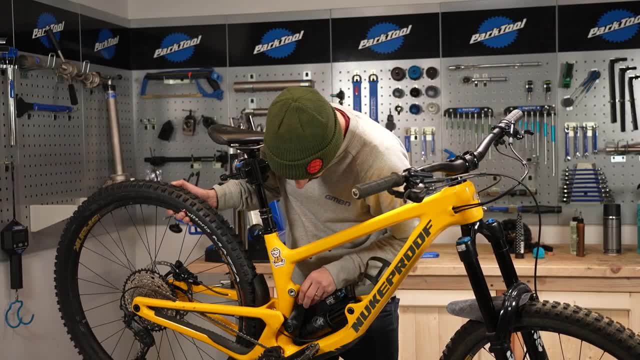 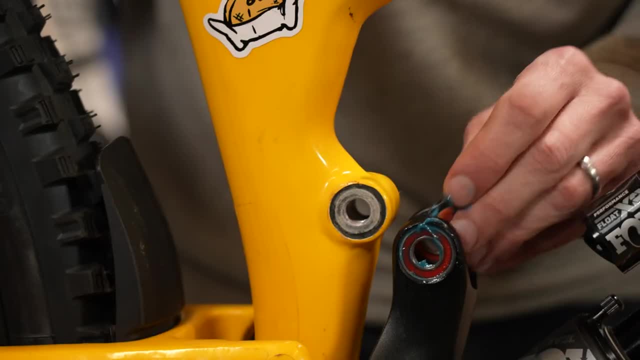 so I'll just put a bit of grease around the outside to make sure they're a bit better sealed and away I go. Top tip here if you've got some of these little spacers that are kind of awkward to fit when you're putting it all back together. 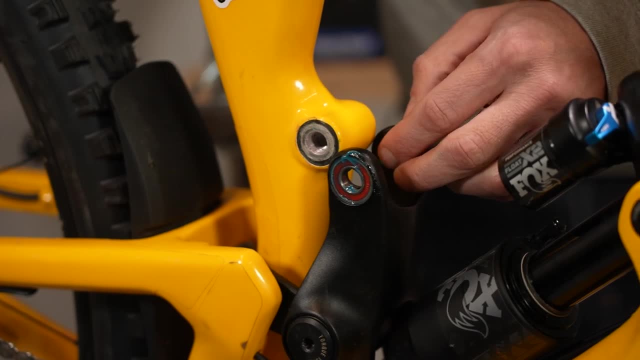 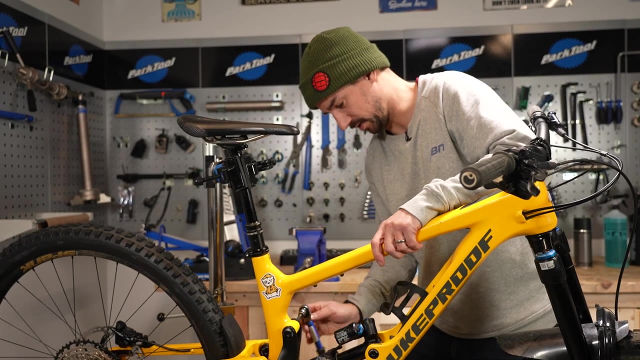 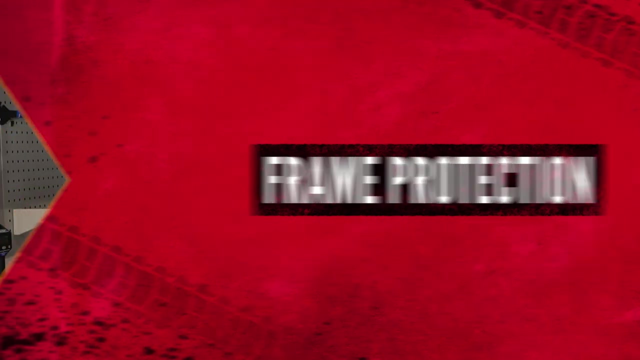 use a bit of grease as glue and then it'll stick there, so you don't need four sets of hands to do one job That doesn't feel tight enough. Prevention is always better than a cure, so if you've got a brand new bike, 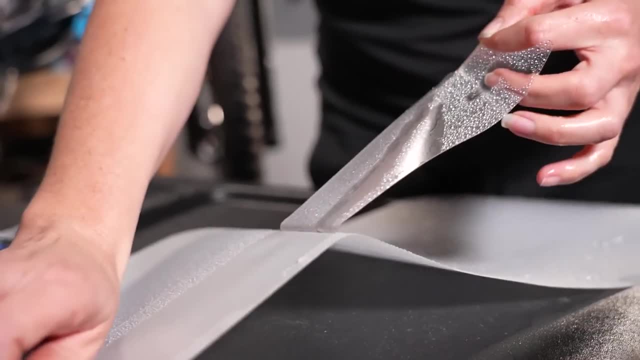 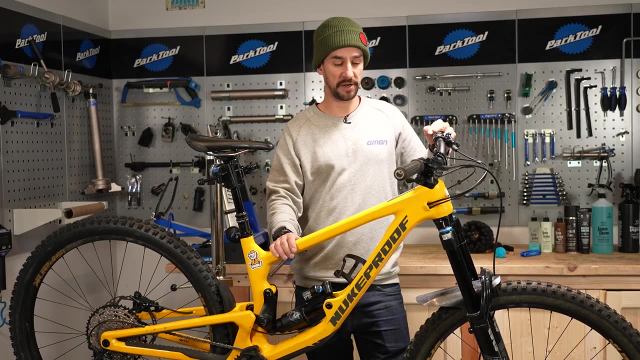 then it's worth thinking about getting a frame protection kit. so a lot of these are invisible, so you can't even tell your bike's got this thin film on there. You can stick it on a bike even though it's not brand new. 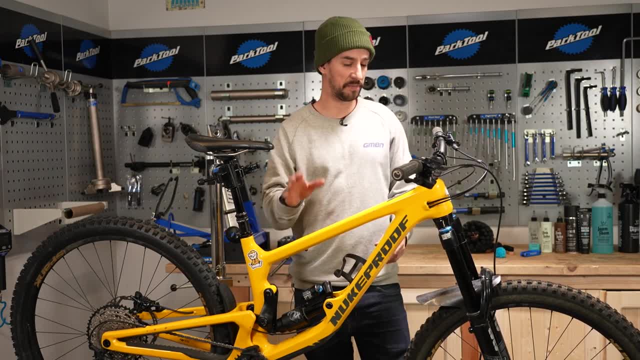 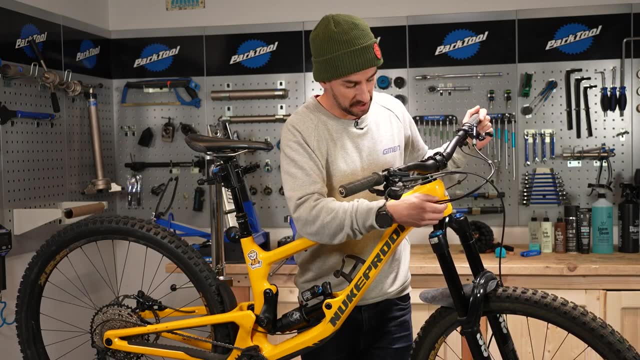 you have to make sure you give it a really good clean and obviously there might be some marks on it already, so you'll lose a bit of that. You'll get a bit scratched up before you put it on, but you can get these extra bits to go on cranks. 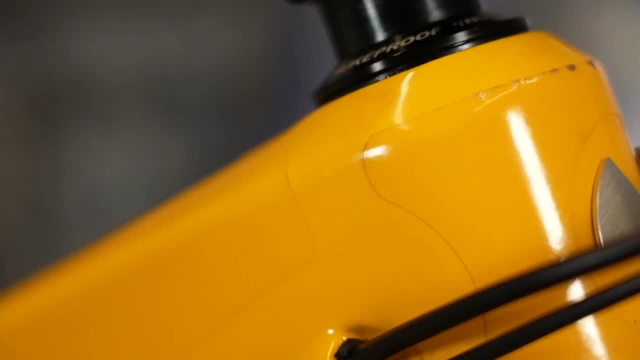 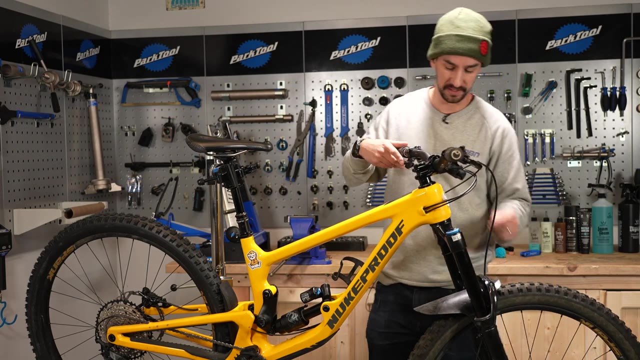 on areas of cable rub What I like to do on a fork. if I stick one of these muggers on with zip ties, these can actually scratch them up a little bit. so get a bit of electrical tape underneath there, It's gonna save it. 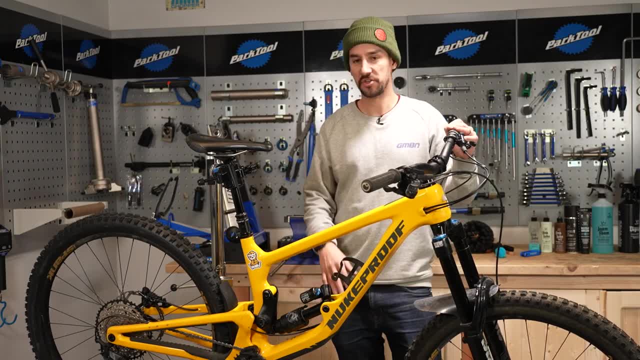 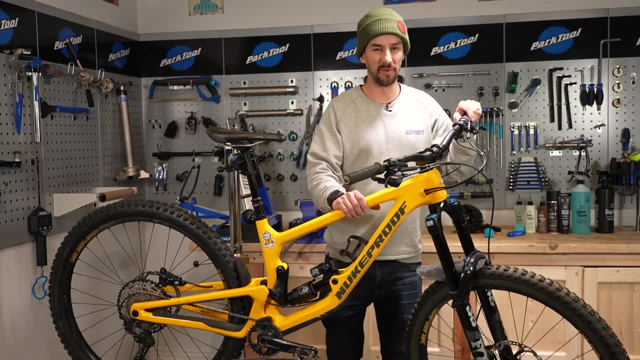 If you want to take it off in summertime, your fork's still gonna look immaculate, so trying to stop it from getting scratched up is gonna make it look new at least. Lastly, I've found that a bike can get damaged more often than not in transport. 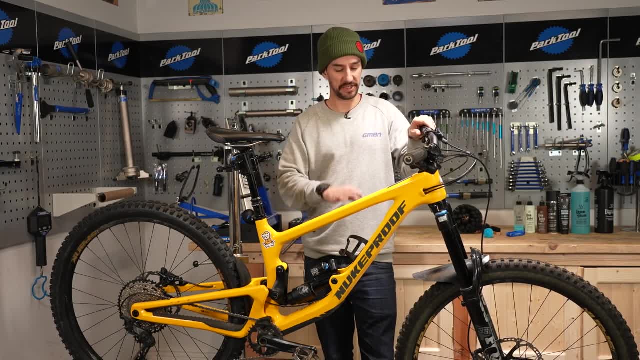 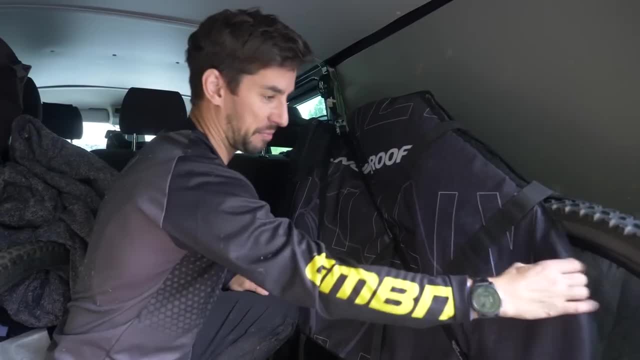 so on the back of the car, in the van, if you're flying with them, make sure they're padded out nice and soft. In the back of my van I've got loads of blankets to cover it up in case I stick other bikes against it. 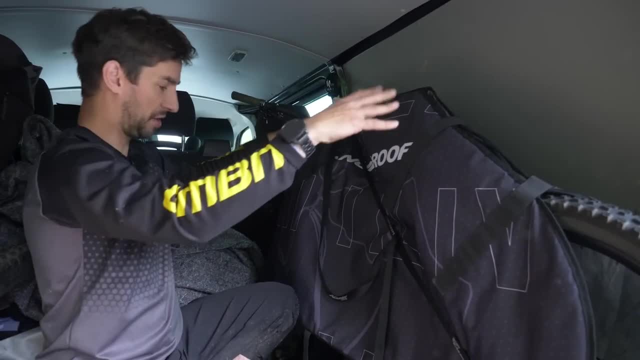 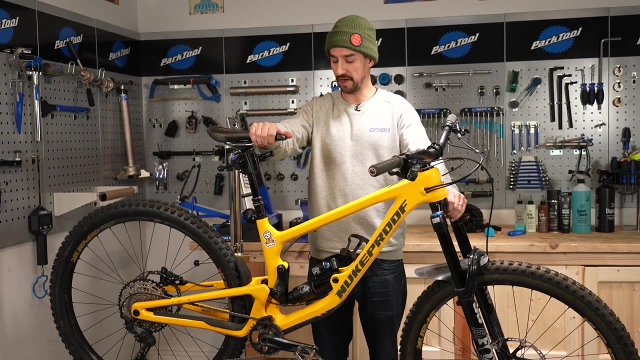 because if you're scratching bikes it doesn't look good. but also if you're scratching your fork leg, then you might need to do a bit of work to that to repair it. So there's my tips for keeping your bike feeling longer. 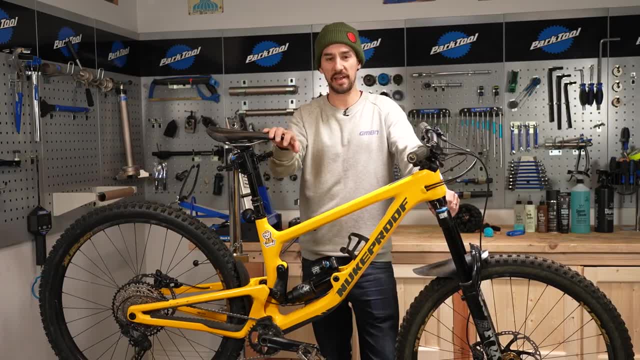 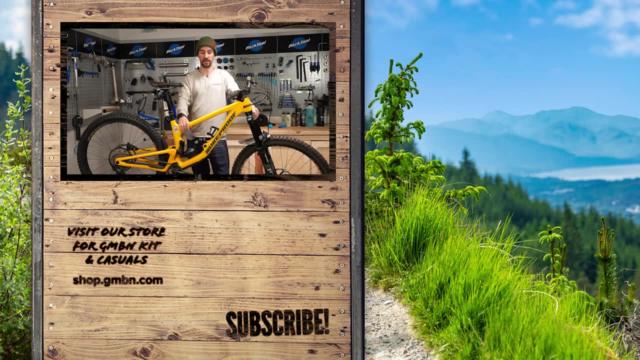 and looking newer for longer, should I say. Also, I think, if your bike has been a bit worn out, don't forget that putting a new set of tires, grips, putting some new bearings in, can make that bike feel like new anyway. so yeah,